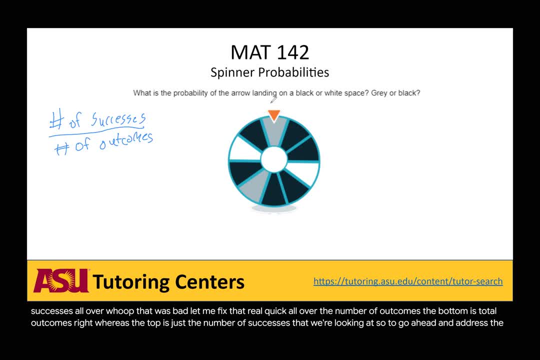 looking at. so to go ahead and address this question, what is the probability of the arrow landing on a black or white space? first off, what we're gonna do is count up all of the spaces on this spinner right. so we have one, two, three, four, five, six, seven, eight, nine, ten. so we have ten spaces right, and what they? 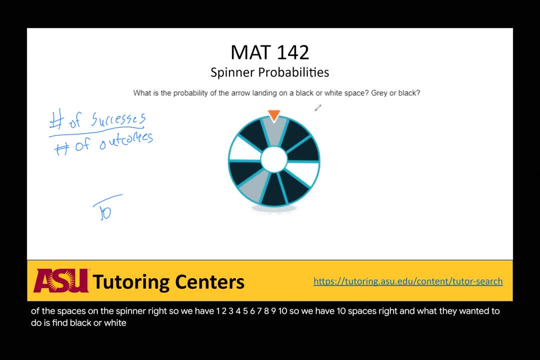 want us to do is find black or white is considered a success in this case. right, so let's count up all the black and white spaces so we have one, two, three, four, five, six, seven, eight. so that means there is an eighth, tenth, or we can reduce this down to four-fifths. 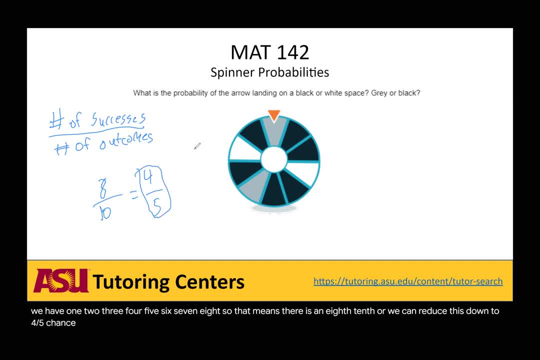 chance that we will spin the spinner and it'll land on either a white space or a black space. Now what they want us to do is find the probability of it landing on either a gray or black space. So it's literally going to be rinse and repeat. So let's count up all the 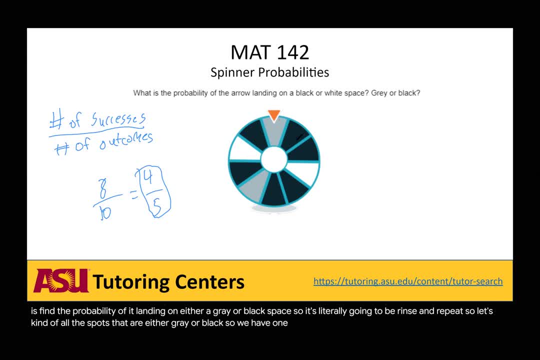 spots that are either gray or black. So we have 1,, 2,, 3,, 4,, 5,, 6,, 7,, 8.. Eight as well, So we have eight-tenths again, which we just said can reduce down to four-fifths by dividing by two, and that'll. 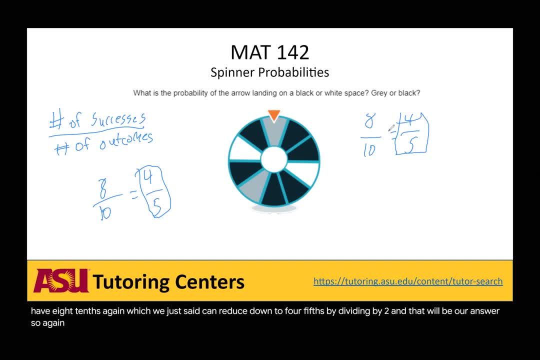 be our answer. So again, the name of the game, again with like, really all of these kinds of applications, is to one, make sure that you know already what is considered a success, right And generally you'll find that in the problem of any spot where they ask for what is the probability of. 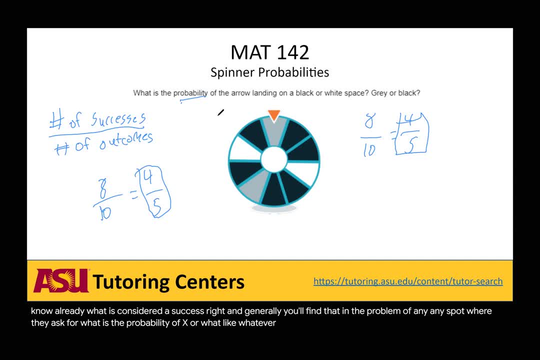 X Or what, like whatever scenario that they're looking for, right? So in this case, what is the probability that it lands on a black or white space Instantly? you should think: okay, so black or white is considered a success, Everything else is considered failure, And that's. those are the. 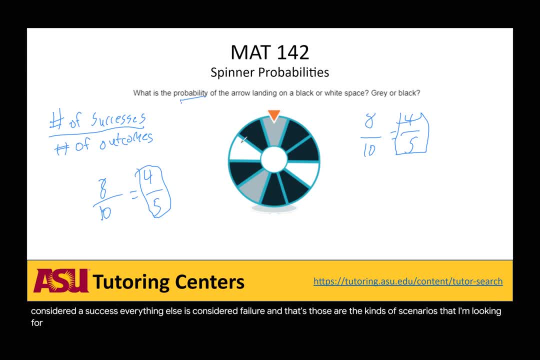 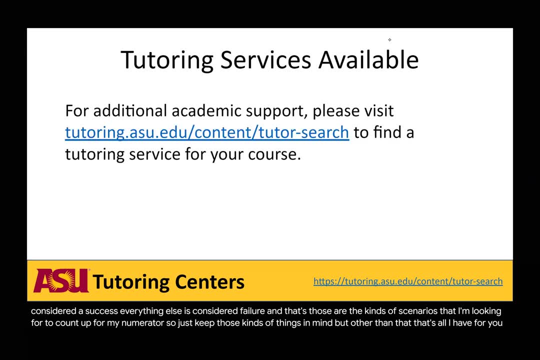 kinds of scenarios that I'm looking for to count up for my numerator. So just keep those kinds of things in mind. But other than that, that's all I have for you. So if you have any other questions, go ahead and check out that link.